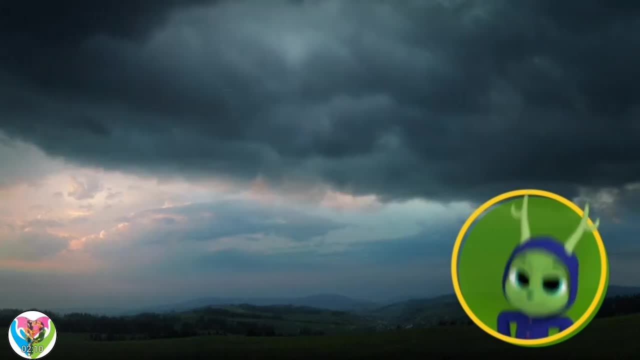 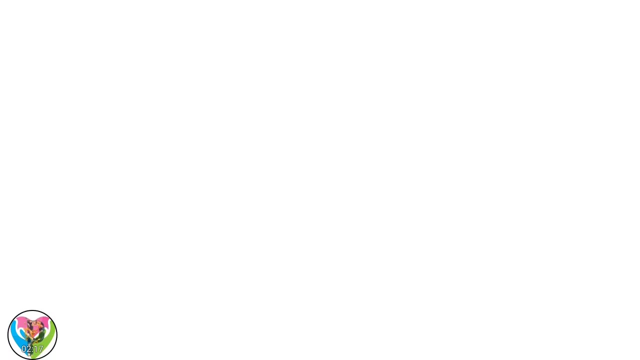 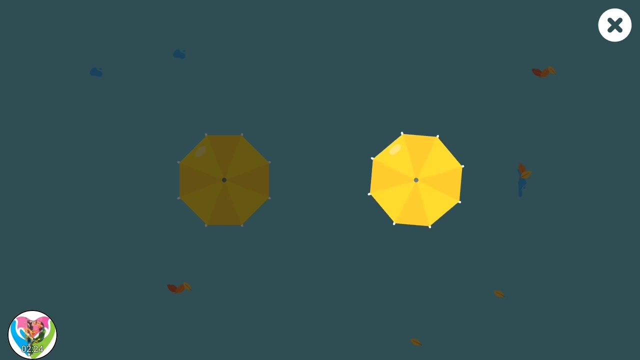 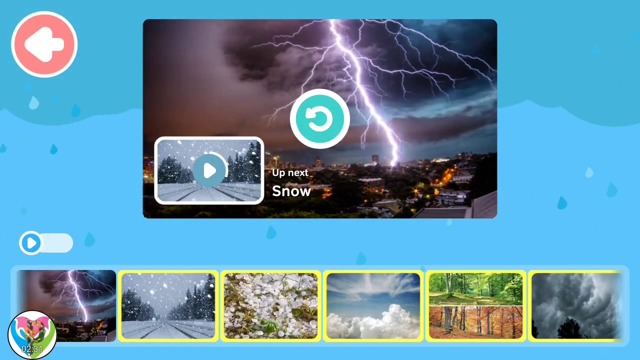 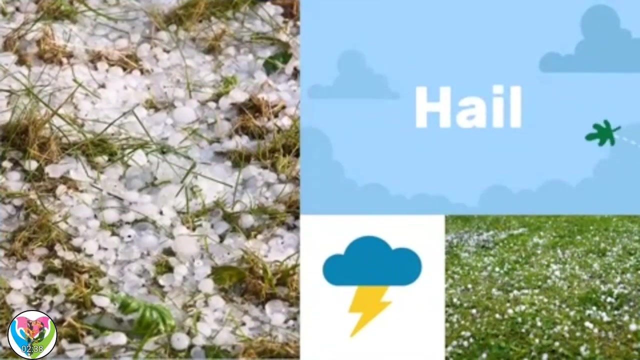 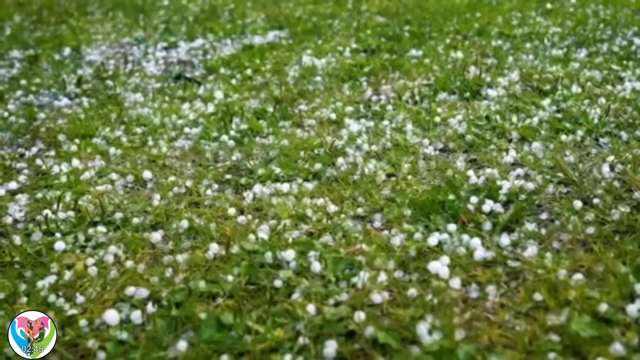 Just call me Electric Chester Zap. Now let's test your memory. Find a matching pair Hail. Hail is a form of precipitation that falls from the sky. Is that hail? It is Gorby. I've never seen hail before. 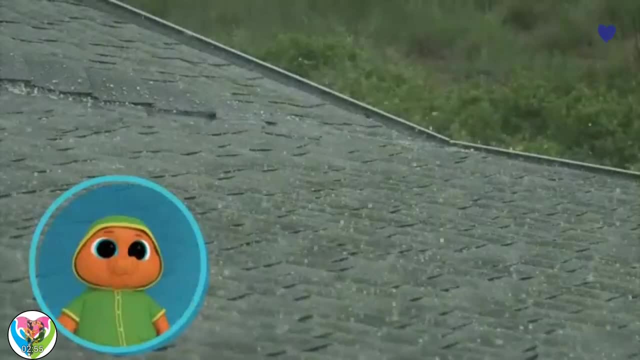 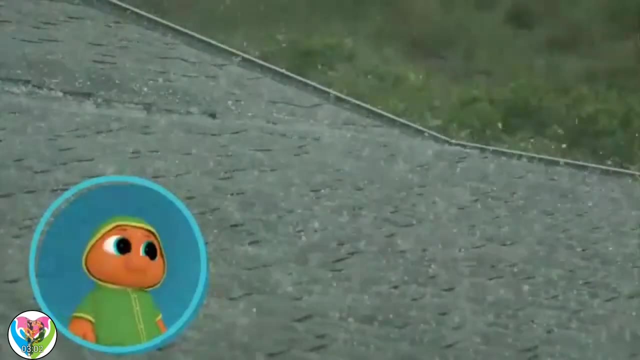 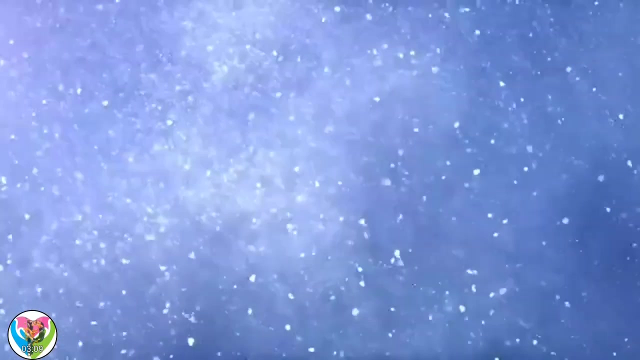 Hail made Well. precipitation is the name given to liquids and solids that fall from the sky, And there are different types of precipitation. When water falls, It's called rain. snow is a light, fluffy, solid form of precipitation. 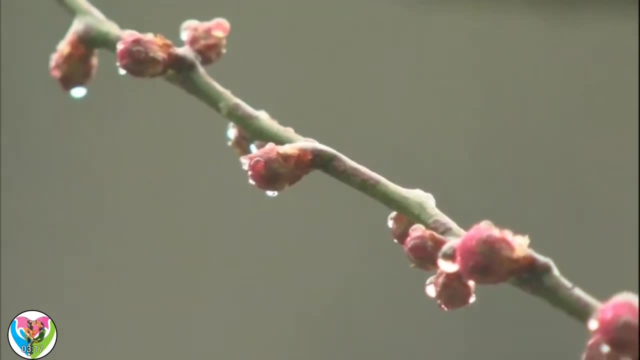 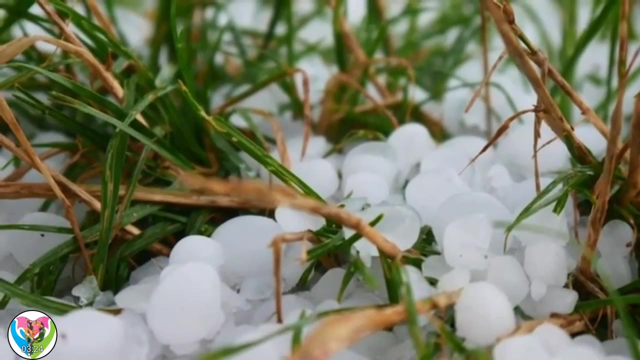 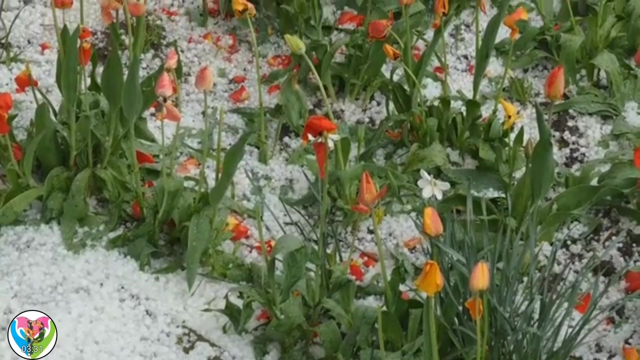 And during winter storms, the droplets of rain can freeze. That's called sleet. Hail is a form of frozen precipitation that's usually larger than sleet, And while sleet usually falls in winter, hail can fall in spring and summer. 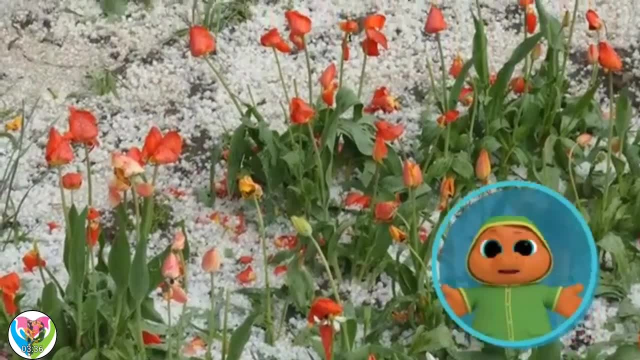 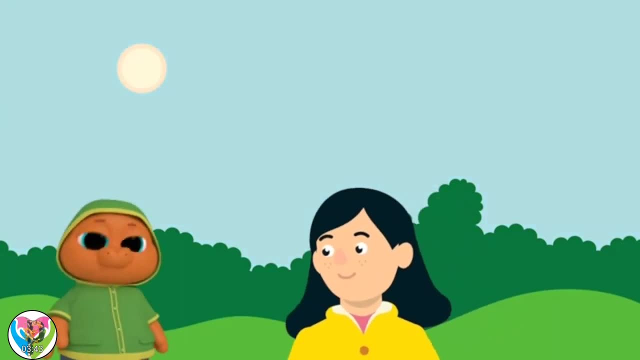 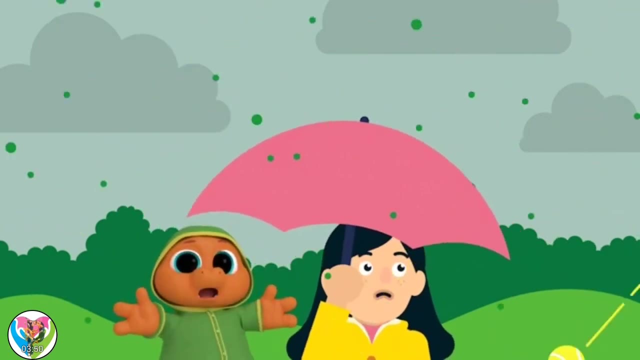 You have to be a bit careful with hail Gorby, Why Usually hailstorms are small, But sometimes they can be as big as peas, Like frozen peas. Sometimes they can even be the size of tennis balls. Tennis balls. 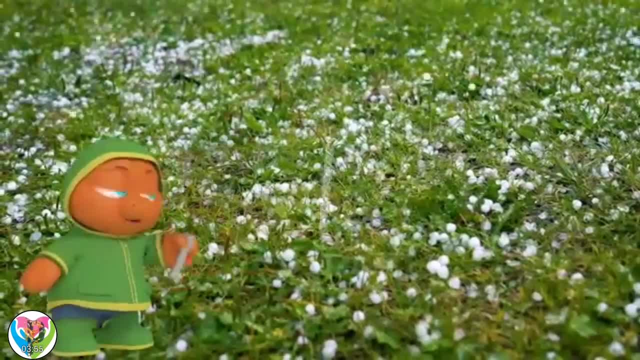 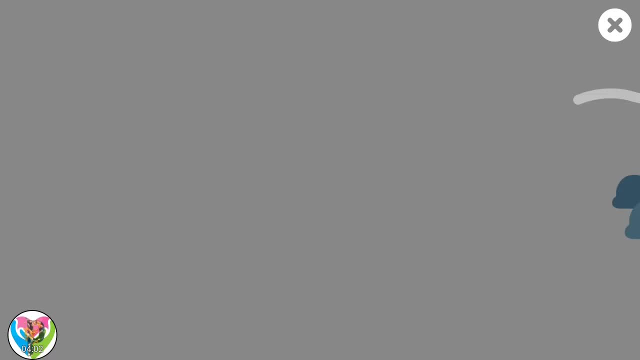 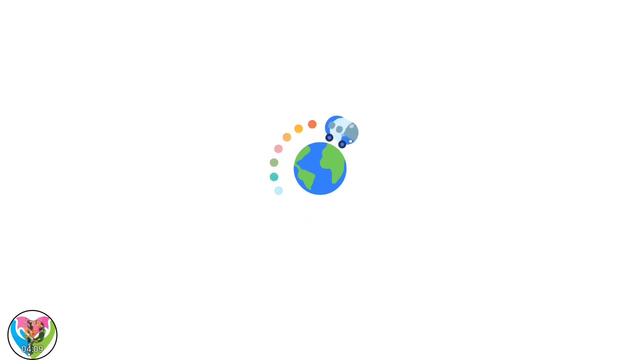 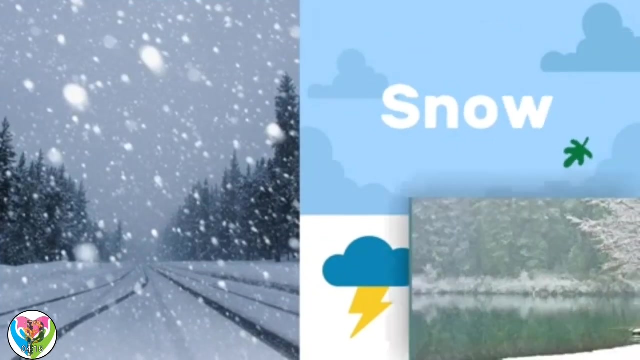 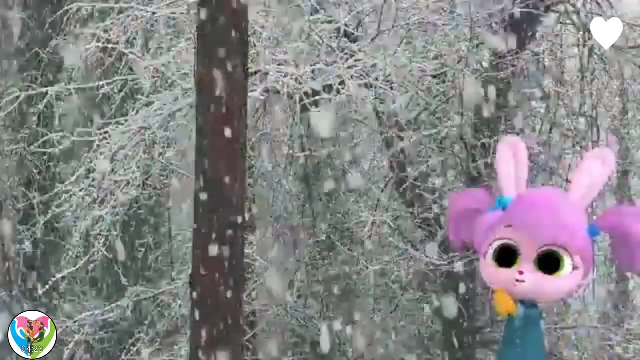 Hold on, Bring it on hail. I'm ready for you. Now let's test your memory. Find a matching pair Snow. It snows in many places where the temperature drops below freezing. I got one. I got one. 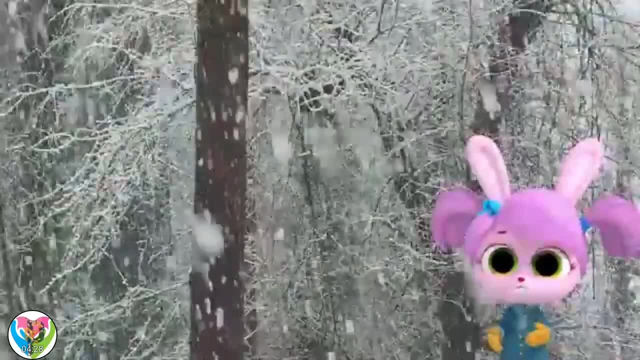 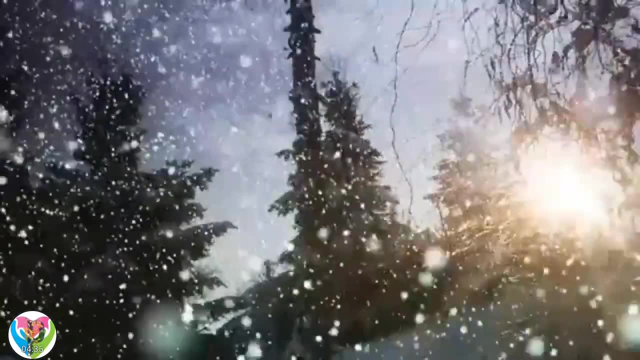 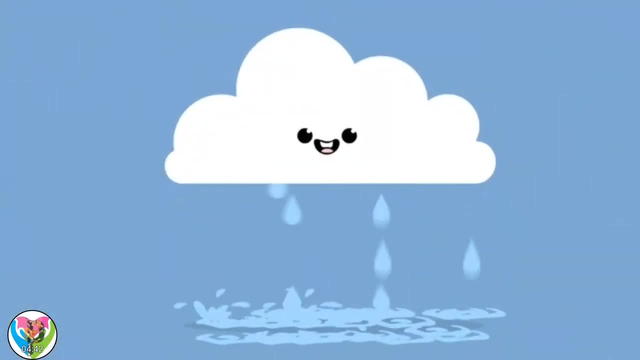 It's gone. Snowflake has melted into a drop of water, Willow Water. Snow is made from frozen water crystals. It's a type of precipitation Sounds complicated. Any kind of water that falls from the sky is precipitation, whether it's rain or hailstones or snow. 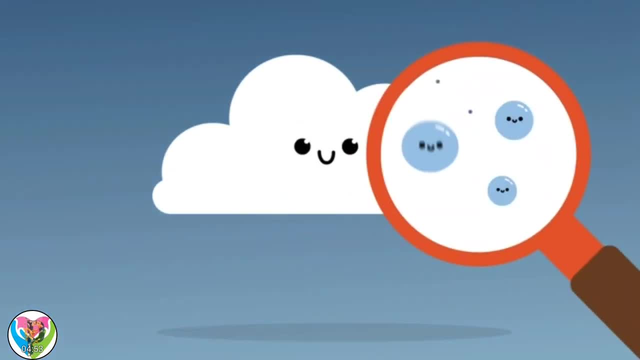 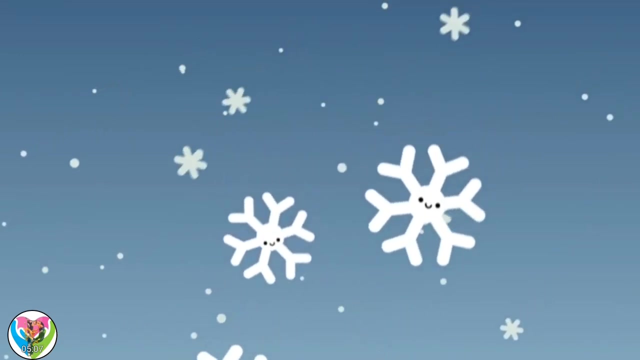 Up in the clouds there are droplets of water. When it gets really cold, those droplets freeze around tiny bits of dirt or dust in the air To become snowflakes. The snowflakes grow until they're so heavy that they fall to Earth as snow. 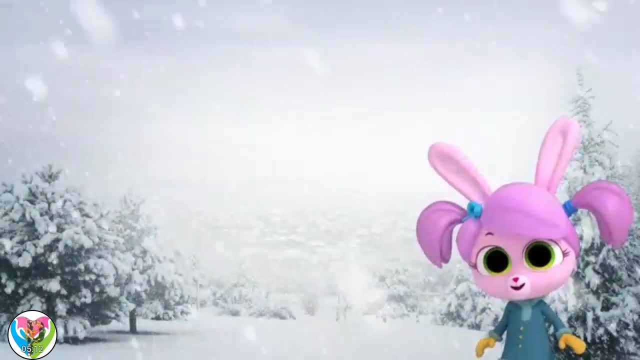 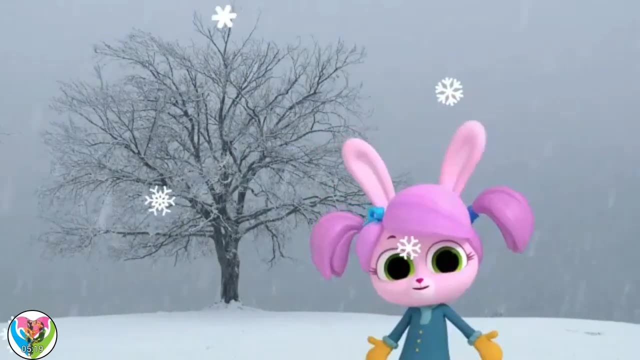 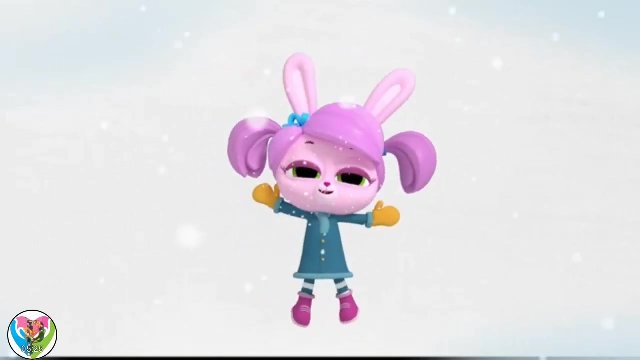 Amazing. What's more amazing is that, even though each snowflake has six points, each snowflake is completely different. That's it. They're unique, Just like us Polos. Just like us Polos. Just like us Polos, Let's spell. 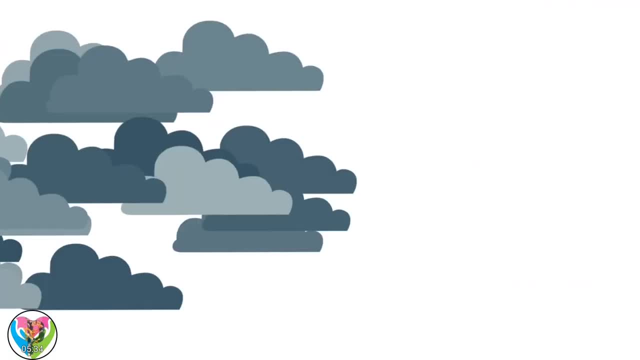 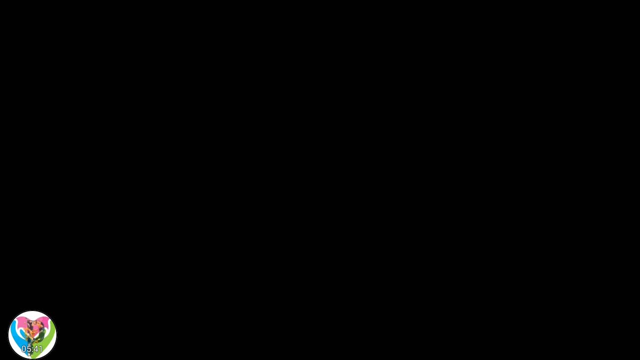 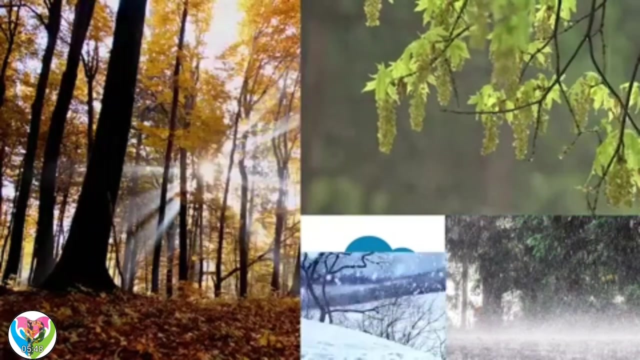 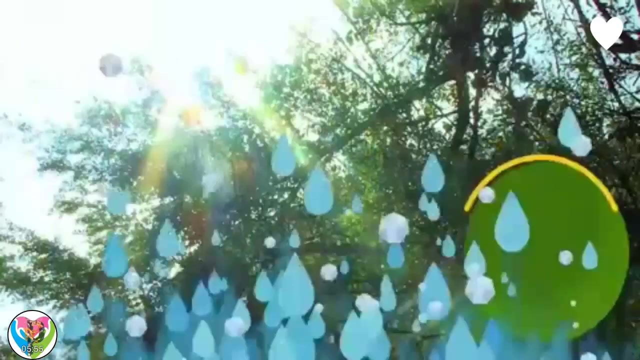 Lightning Seasons. You may have noticed that the weather changes throughout the year. You may have noticed that the weather changes throughout the year. These changes are called the seasons. These changes are called the seasons. Ooh, I know the seasons. Ooh, I know the seasons. 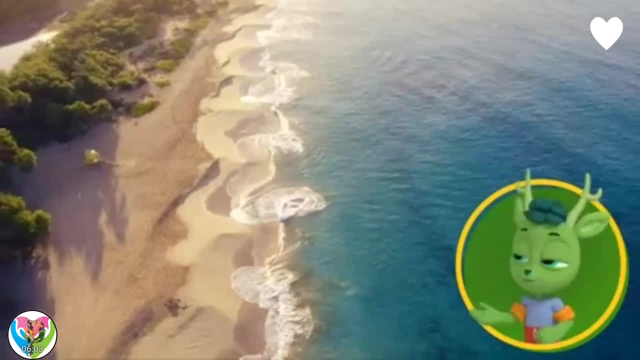 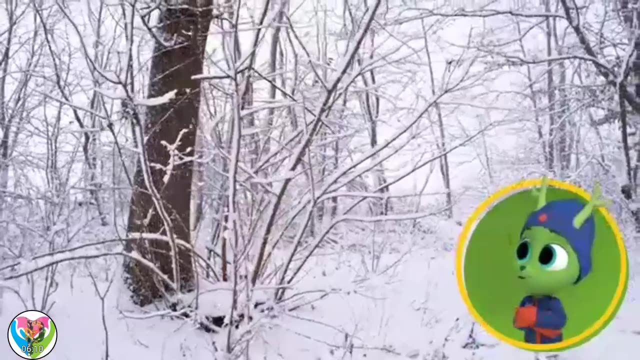 That's Spring. That's Spring Warm and rainy. And that's Summer: Hot and sunny, Windy Leaves falling from trees This Or fall Cold and snow, Cold and snow: That's winter. You really know your stuff, Chester. 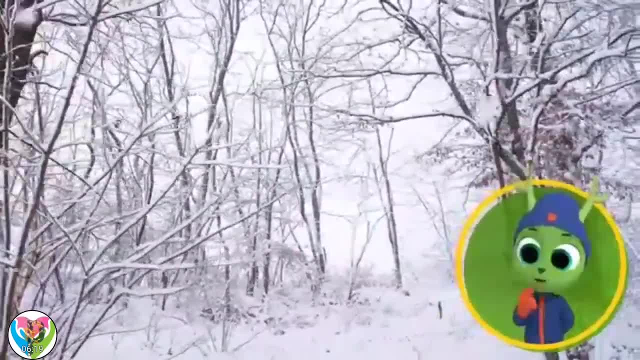 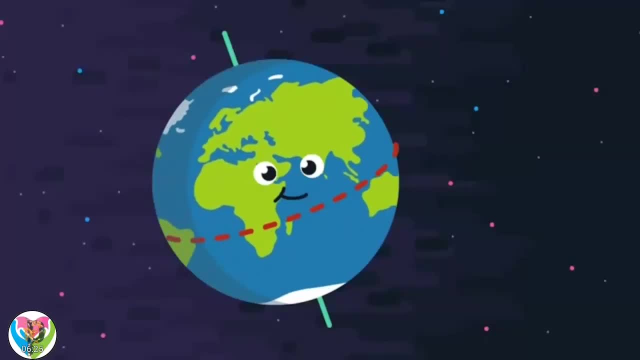 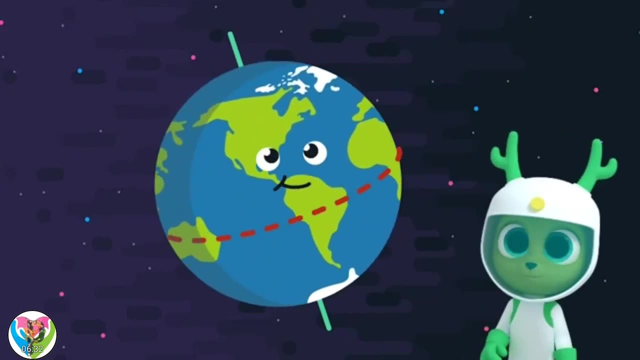 And do you know the reason for the seasons? Is it so we can go skiing and surfing if we want to? Not quite. The seasons are caused by how much sunlight is reaching the Earth. Uh, it's kind of crooked. That's right, The Earth is on a tilt. 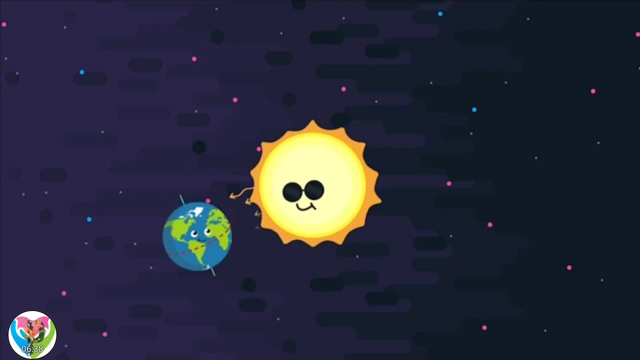 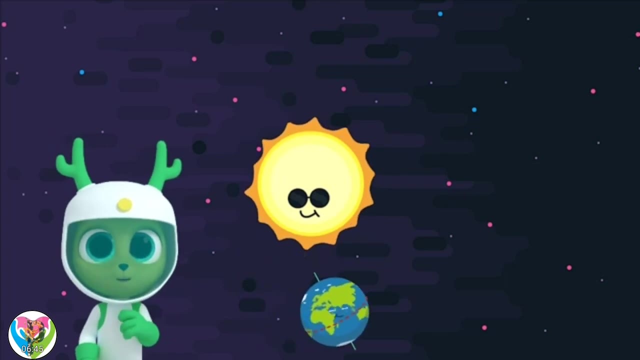 When the Earth goes round the sun, different parts of the Earth get different amounts of sunlight throughout the year. Yeah, the part tilting towards the sun is getting more direct sunlight. So what seasons do you think that part of the Earth is having?